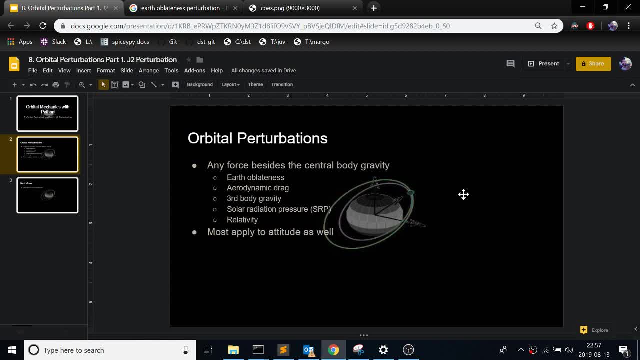 going to be the J2 perturbation. So orbital perturbations, are there any force besides the central body gravity? So earlier, or in all the videos that I've made thus far, you're assuming two body dynamics. so it's just the only bodies that exist are your satellite and the central body. 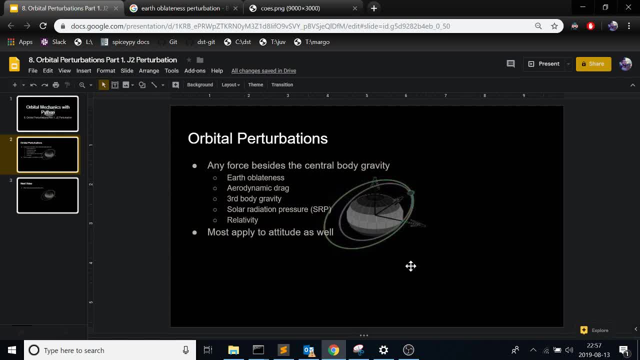 where in real life, this is not true and you're always going to have perturbations on your orbits. Some examples here: earthroblateness, which is J2, and other higher order terms, but basically the fact that earth not a perfect sphere- aerodynamic drag, there's still an atmosphere in space. 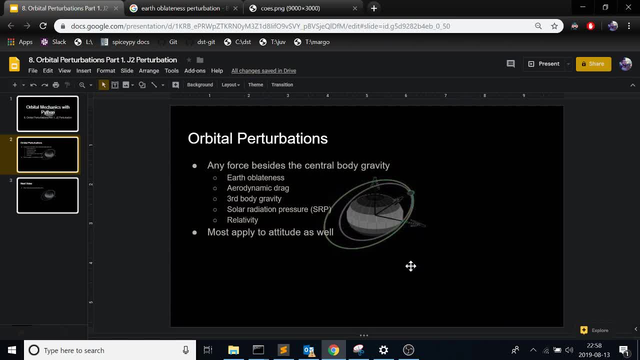 third-body gravity, so the effect of the moon's gravity in orbit and even the sun's gravity as well. So our radiation pressure, the light from the sun. it has no mass but it still has momentum, because- fun with quantum mechanics, I think so it still will give your spacecraft momentum. just a light from the sun. Doesn't affect you too much in earth gravity. but if you get to say orbiting an asteroid, it's a very big deal and you really have to account for it. Then relativity as well. so GPS satellites actually have to account for relativity, otherwise their measurements will. 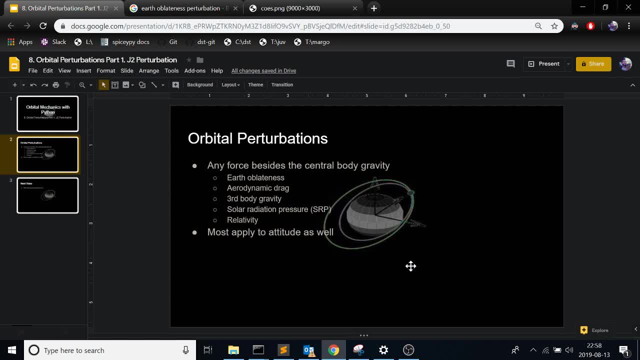 be off by quite a bit fun fact. I might add that later on it's just an equation. obviously relativity is super complex, but at the end of the day, when you put it into orbits, it's just an equation. it is kind of funny. 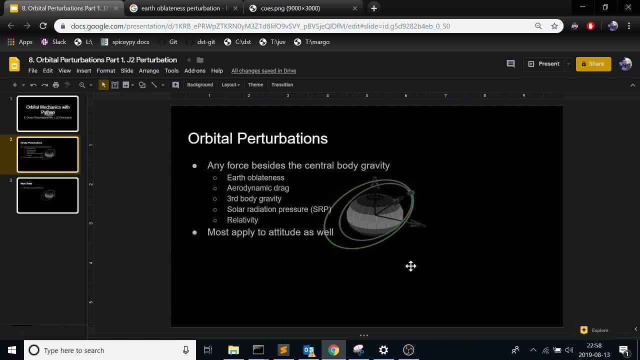 And most of these perturbations also apply to your attitude, which I think actually I'm going to make videos later on down the line about attitude, attitude control and attitude profiles, because I think they're pretty interesting as well and kind of go along with this. but that's just there for now. So I wanted to show the earth, the J2 effect, the oblique effect. I'm going to do a little bit of both of them and then I'm going to show so you can see what happens with the negative part to be the temperature and the disease. but if you're 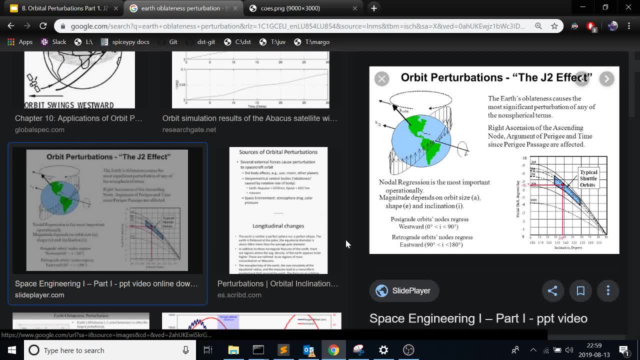 going to put it in orbit. it's better to do the mirror while you're watching this one, So you can actually really get back into the universe. you can actually get a good idea. earth- the J2 effect, the obliqueness effect of the earth. 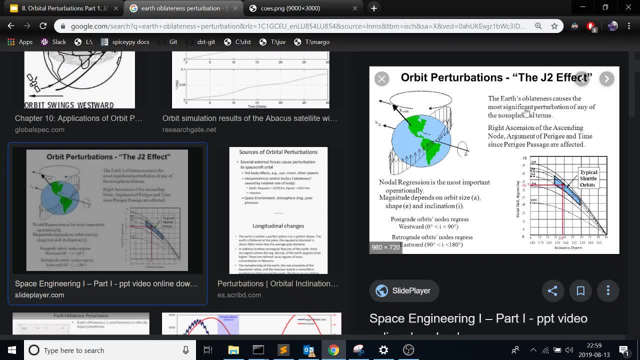 Yeah, the causes of perturbation. yeah, the J2, as I said, there's J2, then there's J3, J4, J5, I think that's like J8 or some large number, but J2 is by far the biggest one. 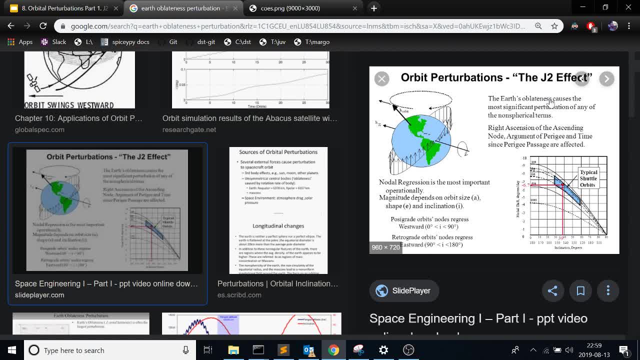 So that's when you're just having a first pass at modeling your orbit. that's where you're gonna use And then what's important here is that right. essentially, in setting node argument of perigee and taxes, perigee passage are affected. 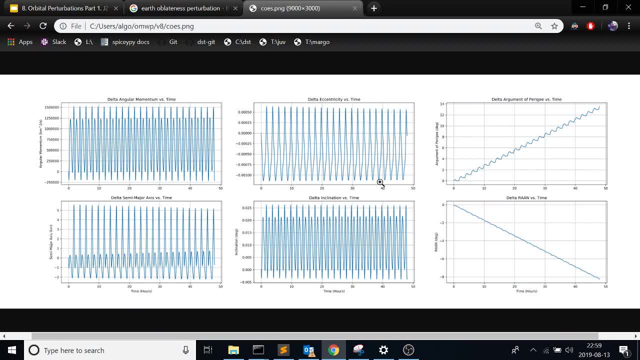 So I can show. I showed this plot in the first video where you can see this is the effects of the classical orbital elements under just the J2 perturbation. So you can see your argument of perigee: over time is increasing like that. 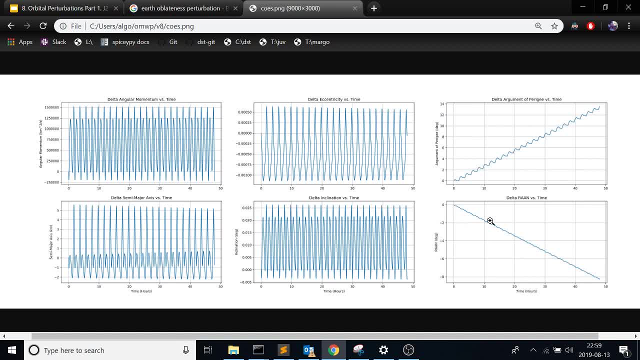 And you're right essentially with setting node is increasing magnitude or decreasing, however you wanna call it, But then the rest of these values are just oscillating. So they're not. it's- yeah, it's- a periodic effect on like a secular effect with these two. 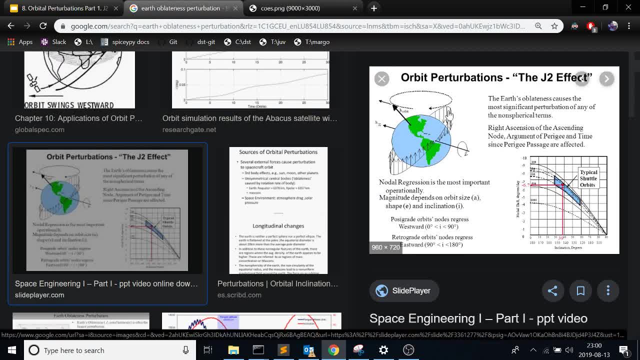 That's kind of what this is saying And you can see kind of a graphic. So when you're up here, you're getting pulled more towards the equator than you are to anywhere else. So the basically where the your acceleration vector. 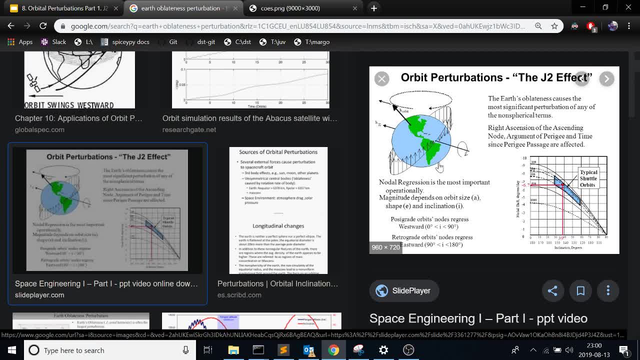 is pointing is not towards the center of the earth, And that's what happens with the oblateness, And I'm gonna post a video on that too, cause I'm just going really quick through it. So you want a more in-depth explanation. 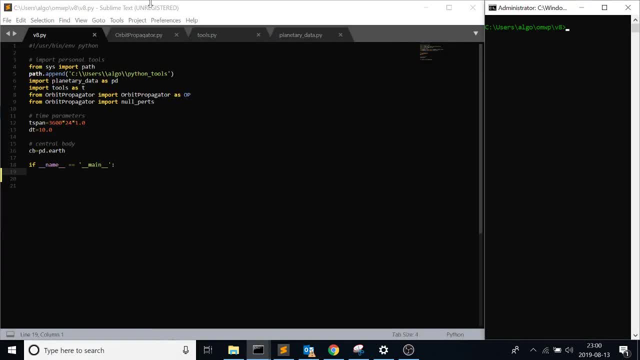 of what's going on there. I'll make sure to post the video. So the software first thing you wanna do is is apply this to the overpopulator class First thing. this might seem a little weird now, because we're only gonna have one value. 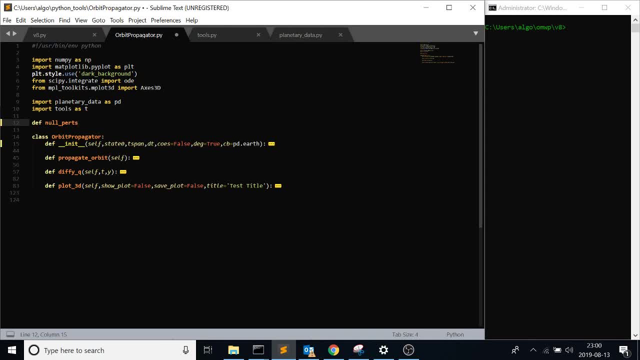 and this video is just gonna be J2 as an honor roll, But later on you'll see that this actually makes a lot of sense And I actually ran the. I'll explain that in a little bit, but I actually ran the memory problems. 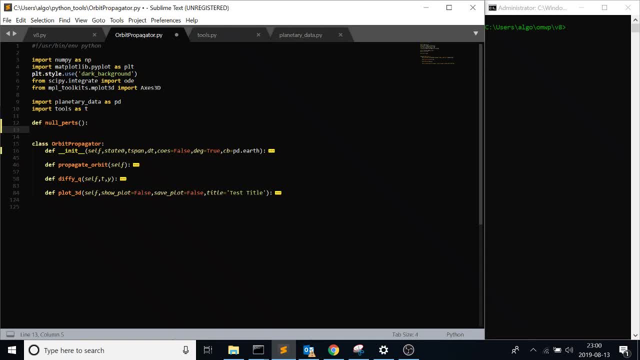 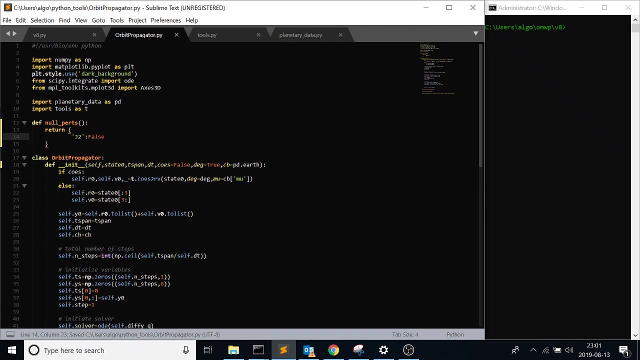 when I didn't make this function, which I guess I'll explain later, cause that doesn't make any sense. Return. so we're just gonna return a dictionary that defines what perturbations you want. So J2 is false. So basically you're gonna call this function. 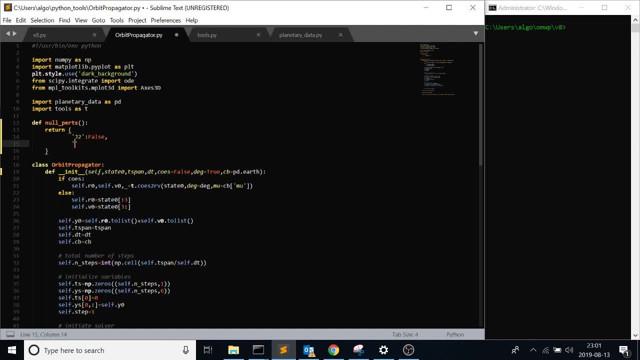 This is gonna give you, so, later down the line, what this will look like. is you say, arrow drag, false. And what are the ones that I say moon gravity? I'll just keep these in here: Moon gravity, false. solar gravity. 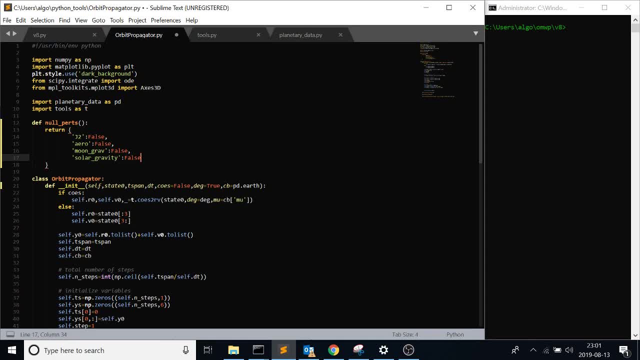 and the reason you wanna have this here is you don't wanna type out every single time you're defining your perturbations dictionary in here. You don't wanna type out every single one, You just wanna load this dictionary and just say I want J2 and just call that true. 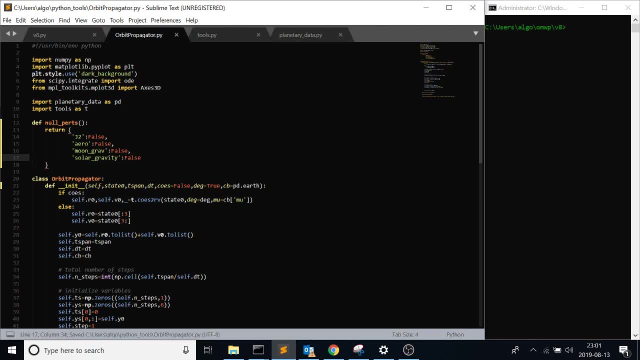 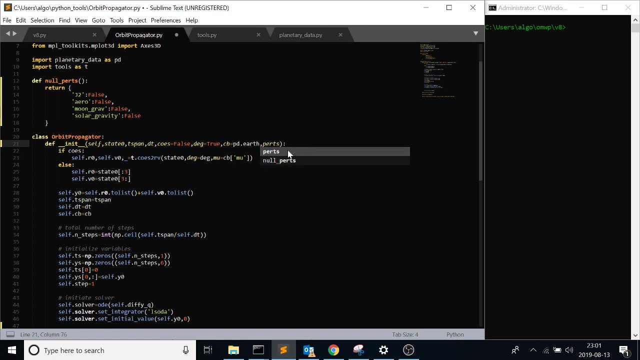 and then just ignore everything else. So I'm actually just gonna leave those there, just because they're all false anyway. so I wanna make a call And then, once you get to your NIP function, you're gonna make it an option. What's it called? 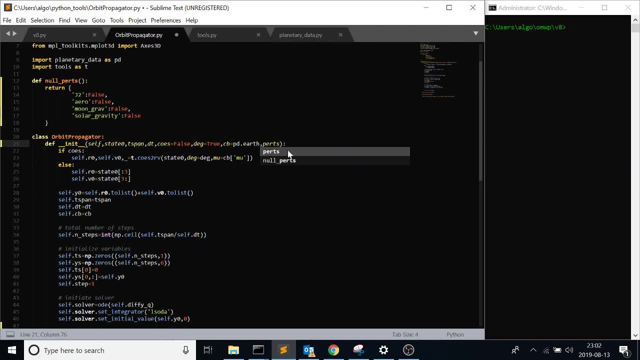 You're. it's not gonna be a argument You have to pass in just because sometimes you don't want perturbation. You don't wanna see a two-body orbit like we haven't done before, So just don't worry about it. So pert equals null pert and it's calling a function. 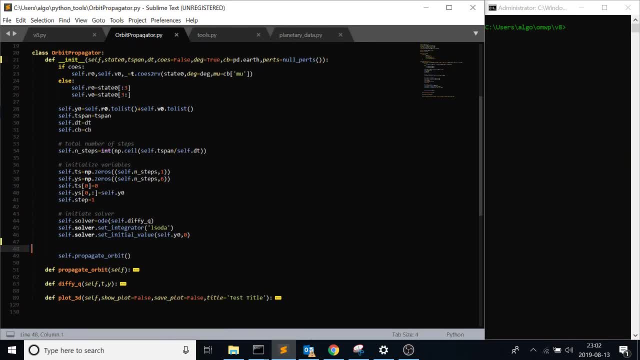 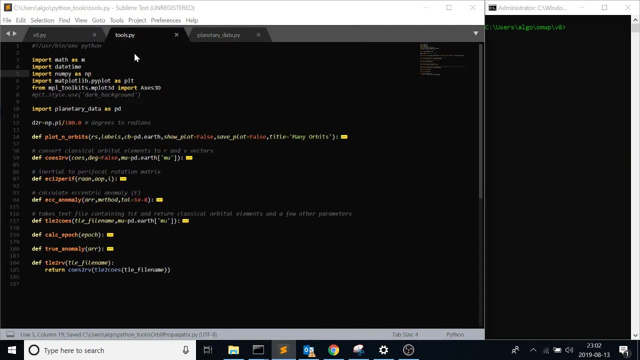 because it's returning this dictionary And then just say: define perturbations dictionary. So I'll put pert equals pert, just like that. Oh shoot, I accidentally closed it. Hopefully I didn't lose that Propagator. okay, so so the pert equals pert. 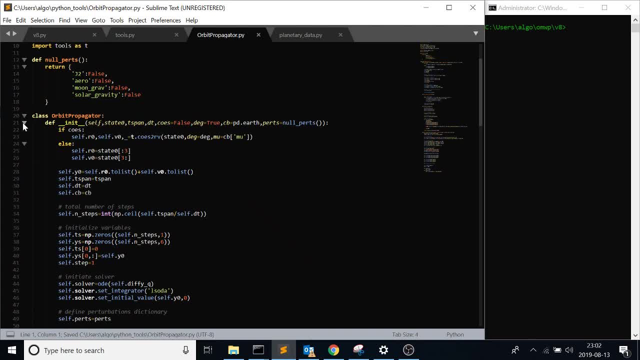 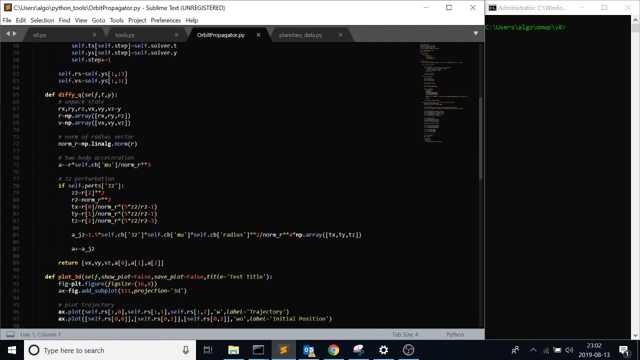 Okay, we've got that. Yeah, so that's the finding it in the NIP function. Just make sure you're calling in and then where it's gonna be called is here. So I already wrote this down because I didn't wanna, kind of again. 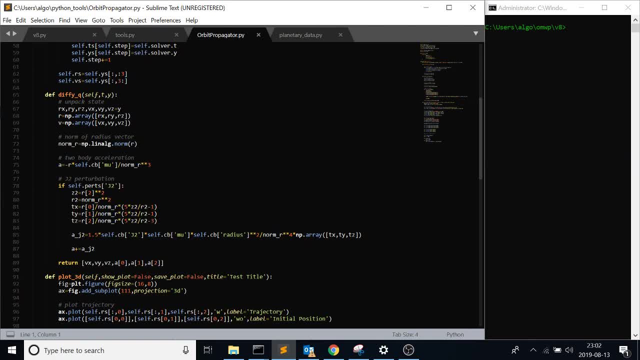 bore you with equations. but what's happening here? So you have seen this: before your two-body acceleration, and then after that you have your J2 perturbation. So if the perturbation is going to be, you know, a two-body, this dictionary, the J2 attribute is at the true. 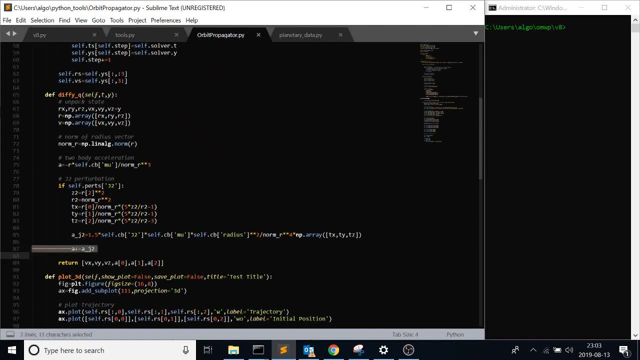 and calculate it and then add it to the acceleration. that's already here. These are all arrays. You can just add them element by element, like that. Again, just equations for the J2 value of the earth. I'll get to that in a second. 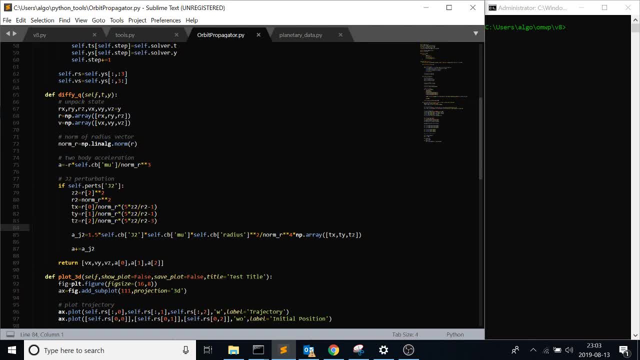 And then mu radius, just an equation. I'll you know, I'll post a video to kind of explain it. That is what you're doing. If you're calling J2 perturbation, run that. If you're not, then just don't add anything to it. 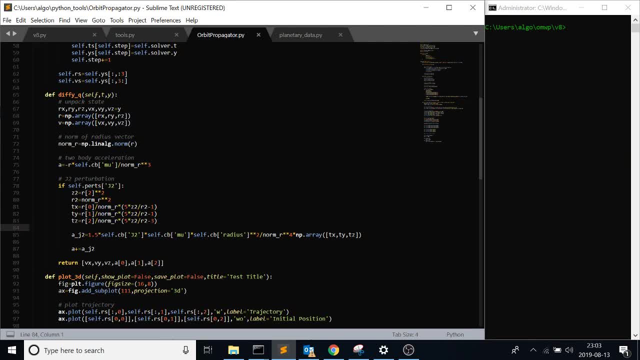 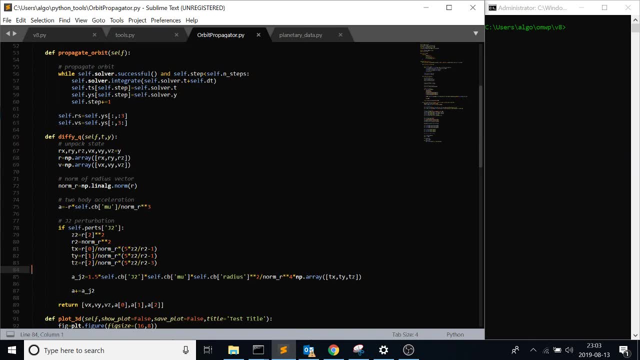 And this is the same as any other two-body orbit. You don't have to worry about it And all you have to do is pass in one dictionary And that's supposed to be kind of just like again level of distraction. Just say I want this perturbation. 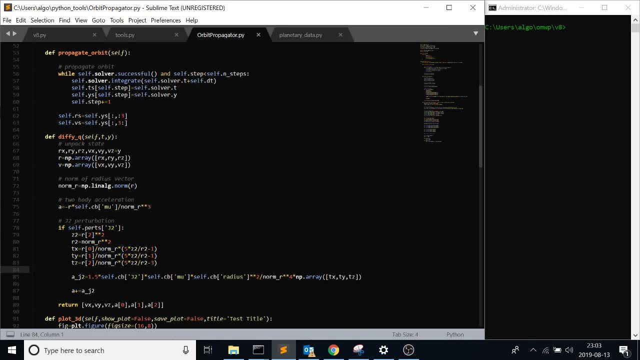 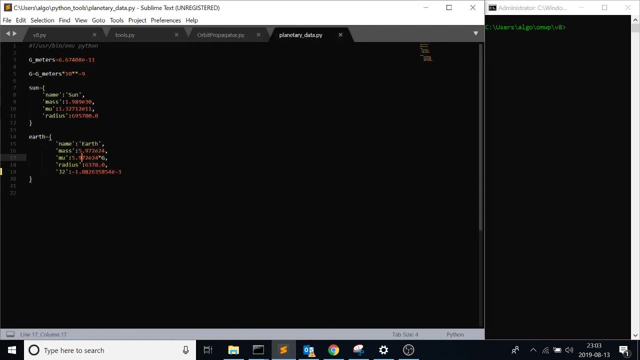 Okay, cool, And then let orbit propagator take care of it. And then, as far as this J2 value, this is another value that you add to the planetary data for each body. This is a J2 value, It's just a number. 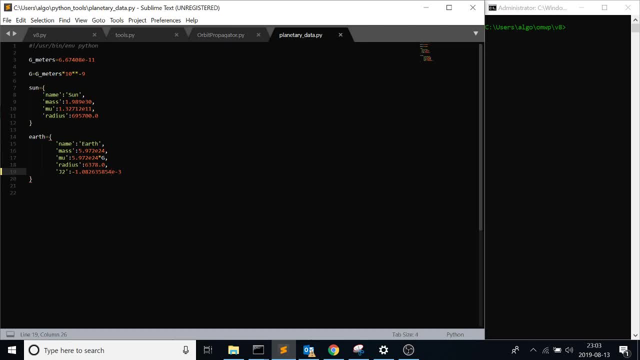 And there's a lot of math that goes behind- how to find this and how to apply it. But again, when you're plugging it in here, it's actually pretty simple: Just have that number. So I think that's good for that. 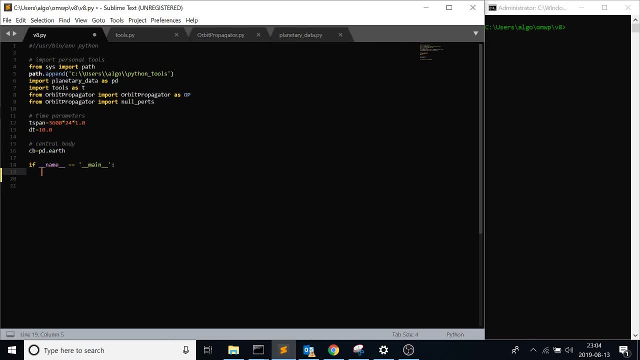 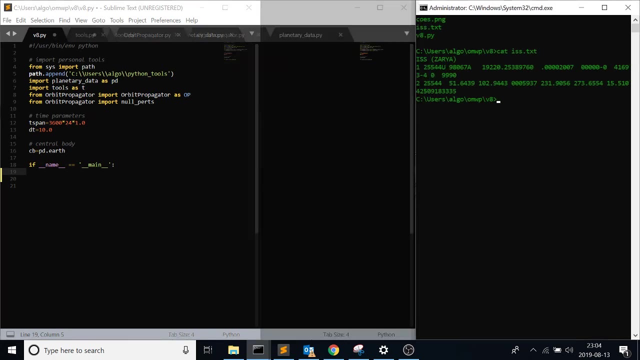 And then we'll get to here. So again, I want to do an ISS example. So in this current directory, I copied over this ISSTXD, which looks like this, like that. So what I want to do is I want to create. 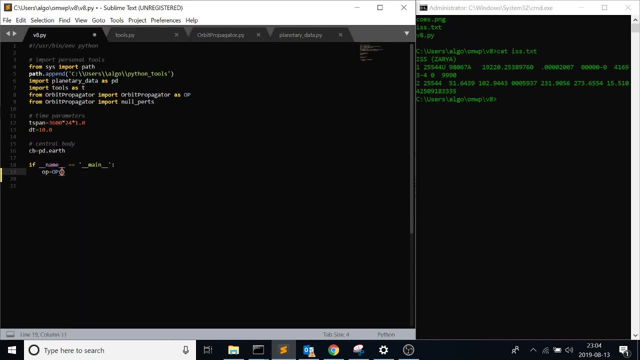 an orbit propagator. class OP equals OP. where we have that, our initial state is going to be dot TLE to pose, because this is a function we wrote, so this makes it really easy. Pass in the file name: ISSTXD. 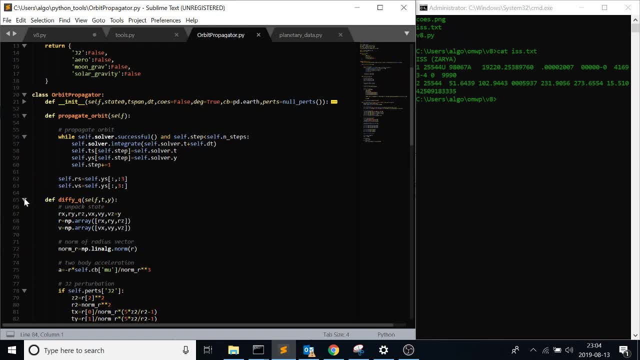 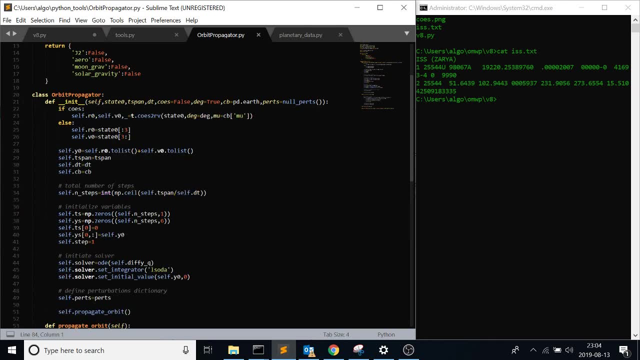 and you're good to go, Yep. So that's the first argument. And then I have to put it in Whoopsies: Yeah, it goes. And then you have to make sure you have degrees equals, true. And then TSPAN DT. 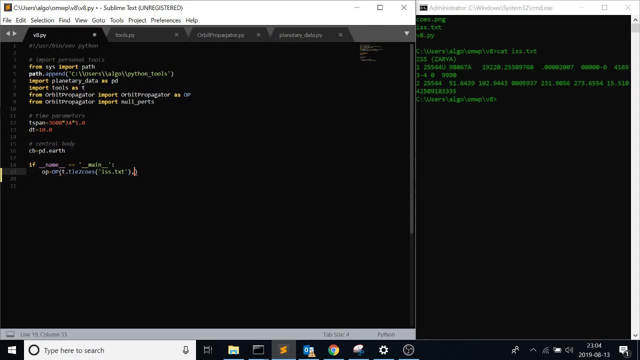 We go TSPAN, let's just say, oh, I have it up there, Yeah, 24 hours, But actually I'm going to make this a bit longer so you can see it. So you can see kind of the effects of 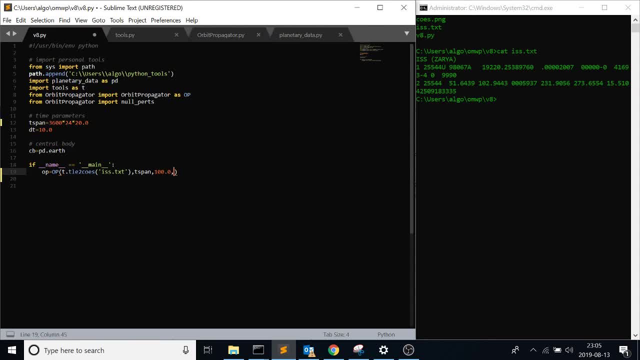 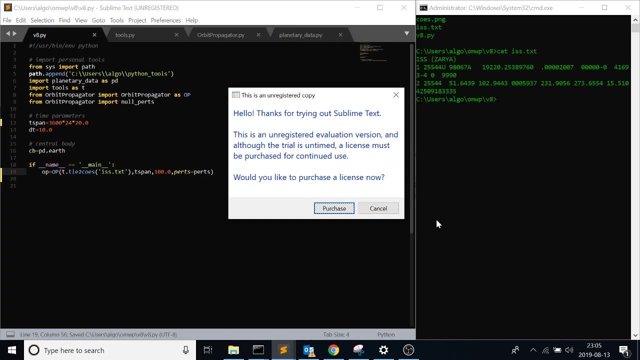 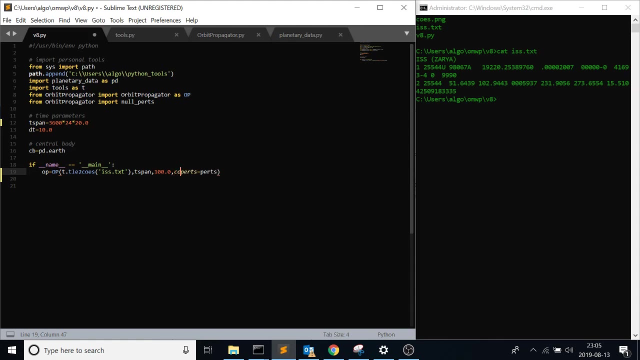 and what's going on a hundred times. And then, oh, and then you say perts, DT. oh, cos equals, true also. So that's perts equals perts. What you're going to do is you're going to define. 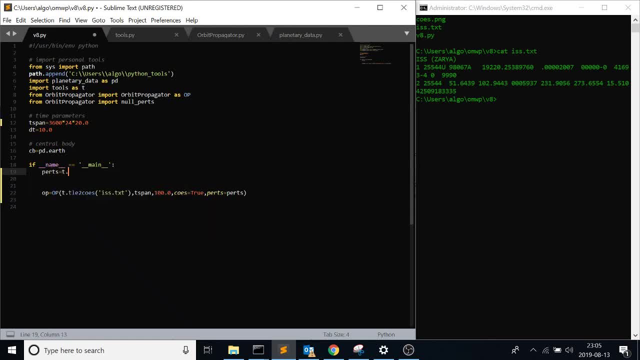 you're going to define this dictionary as: perts equals T, dot null perts or just null perts, because this is a new import you're calling it here. So the import that was before was from orbit propagator in import: orbit propagator. 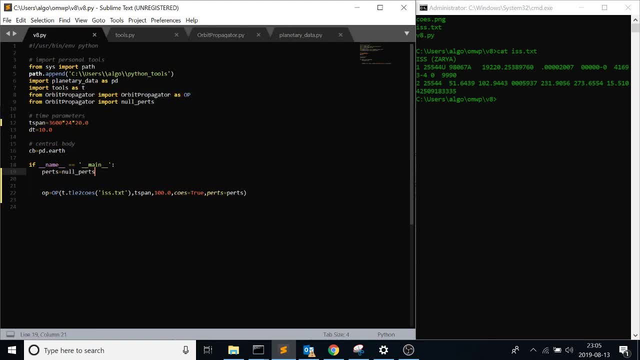 from now it's. And then now you're adding: from orbit propagator import null perts or it's a function, So you call it and then, super simple, You just say: perts J2 equals true, And then you have. 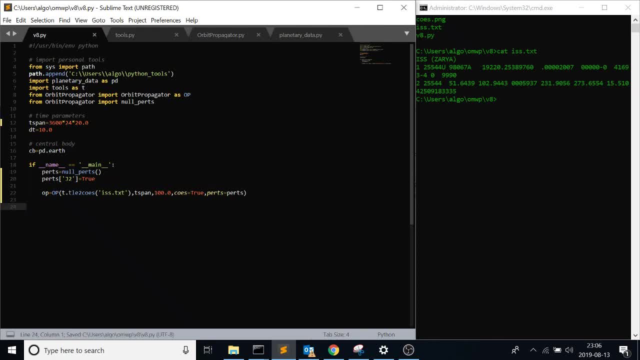 have your J2 turned on And then, if everything went well, as you propagate, orbit is already in the minute function now, so you're going to have to call it plot3D. showPlot equals true. So you have all that. Did I pass everything in? 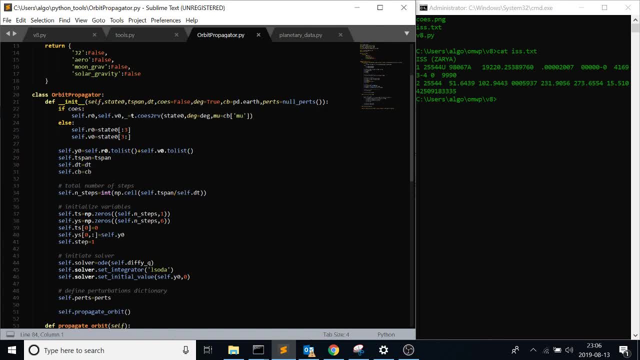 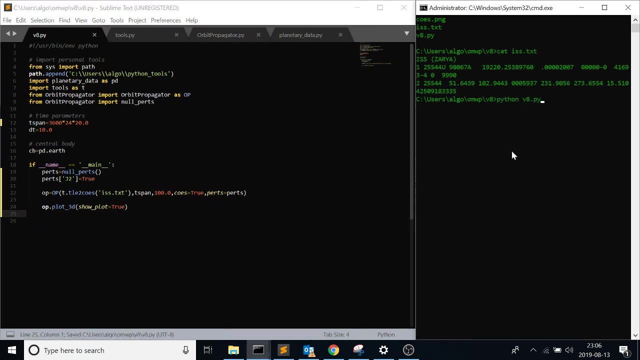 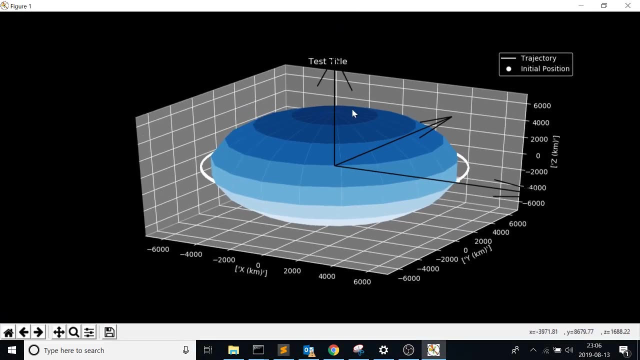 T span, cos, dt, cos tan. Yep, that should all be good. Let's see what kind of errors we're looking at. And it worked Cool. Wow, Another one with no errors. That's amazing. It might be a little hard to tell. 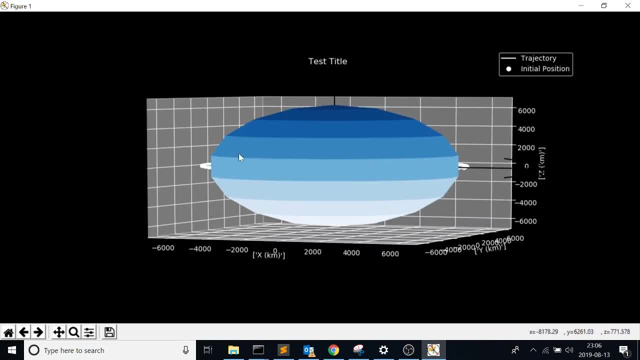 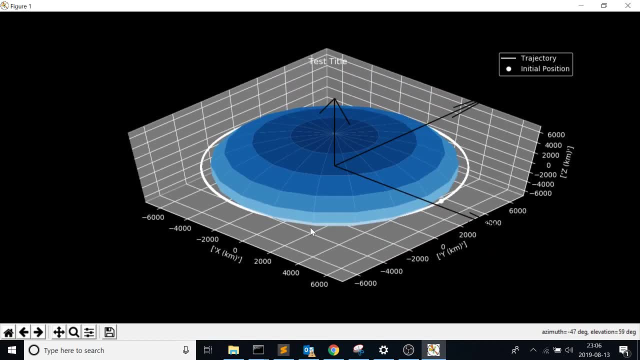 It's a bit subtle, But these lines are thicker than they are before just because there's more passes going through them. It's not just one time going through. so it's making a variation to those parameters, But it's hard to see. 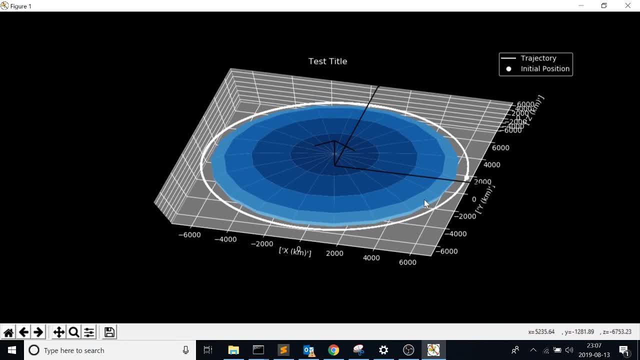 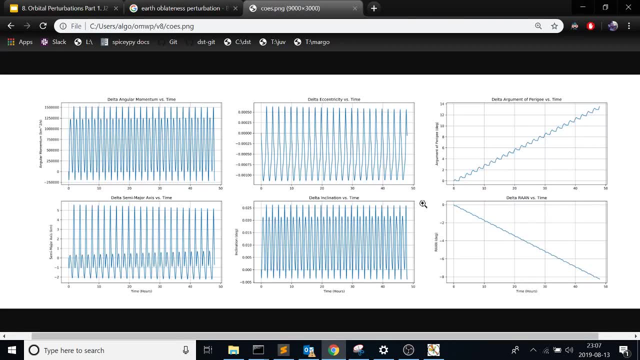 It's hard to see on this scale because the Earth radius is so large. These are the values we're working with, But they do have a variation that is noticeable, as you saw in these values. This is a noticeable effect If, over two days, 48 hours, you're. 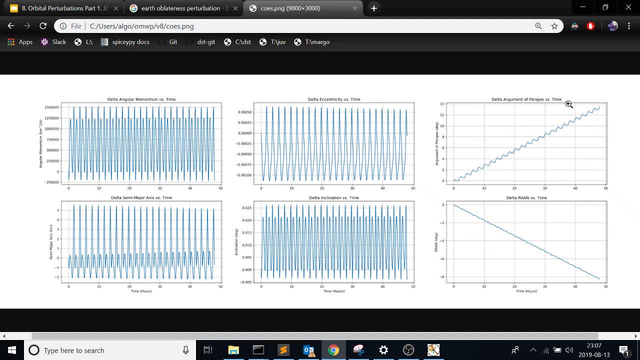 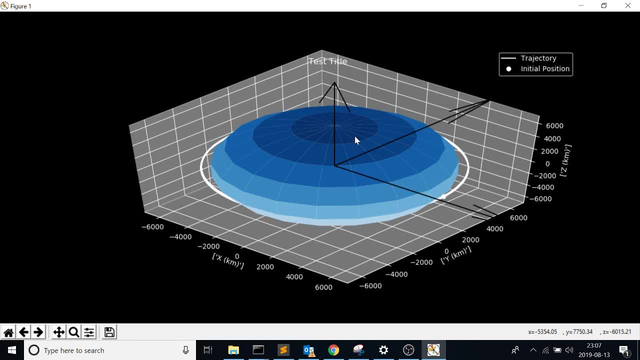 going to get a change in rand of roughly 8 degrees and then a change of argument of perigee of about 13 degrees. So that is significant if you're trying to talk to a spacecraft, because if you think it's somewhere and then it's actually somewhere else. 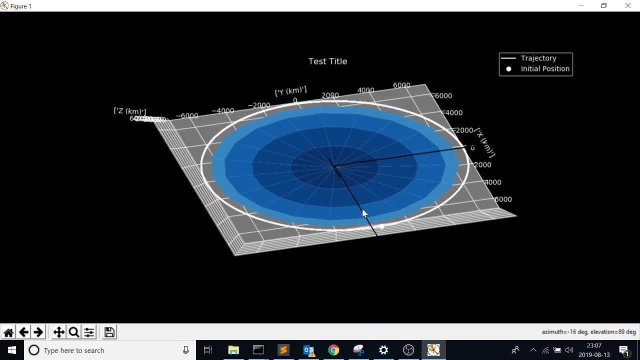 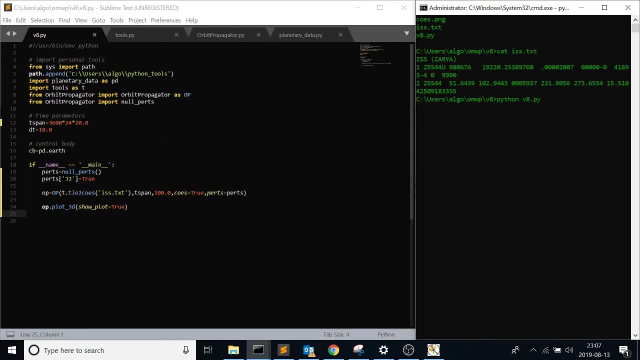 you might not get to talk to it. So this is something that you have to model. OK, And that's about it. for this one, I think I kind of showed you how to implement it And kind of the most important part of this video. 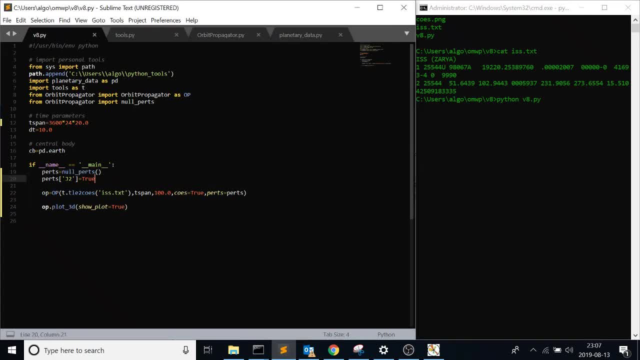 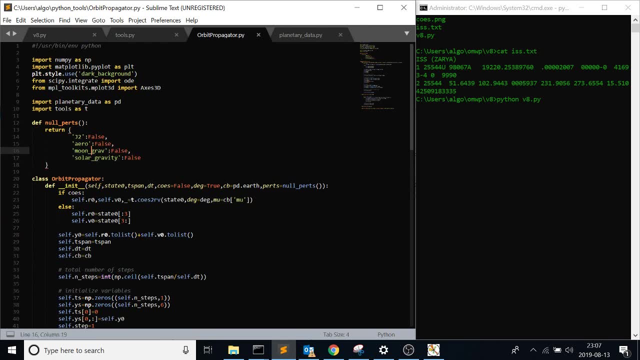 is understanding that this perturbation is dictionary because we're going to build on that. So, as I defined it here again, I didn't use these in this video, but I'll get to the aerodynamic drag kind of term and how to implement that in. 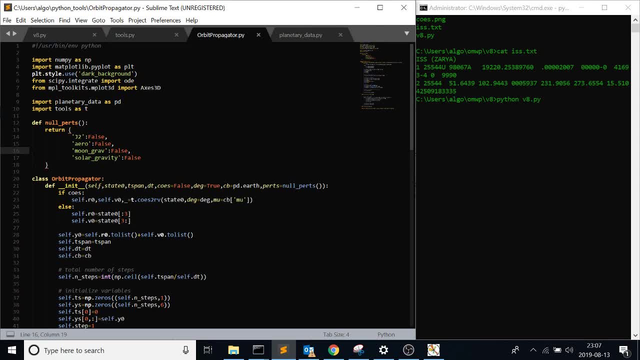 The moon gravity as well the solar gravity. Maybe I'll get to relativity. I don't know. It's not actually too important, Unless you're doing GPS, But that's the kind of important thing to grab here is how to apply this. 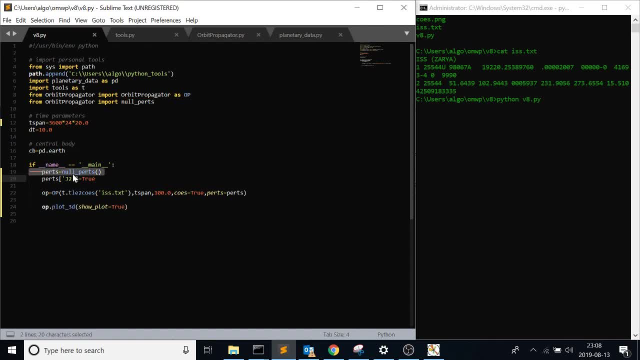 So all you have to do when you're actually calling it is just say: give me a perturbations dictionary and just J2 is true, And then let overpropagator do the rest of the work. So I think that's it for this video. 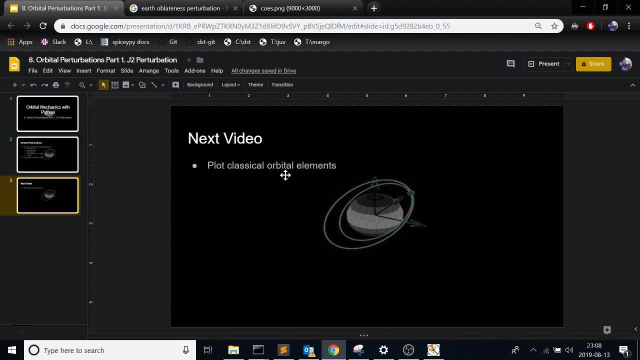 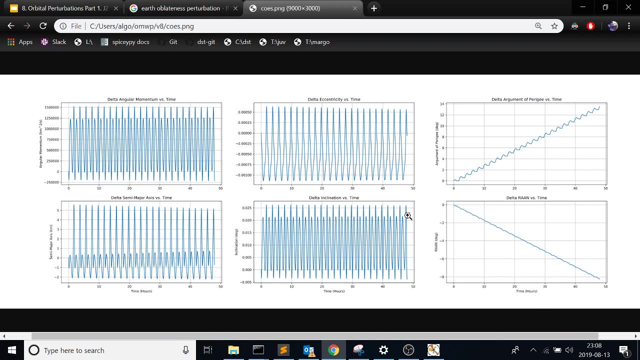 And the next one. I want to go ahead and write that function. Actually, before I write the aero drag function, I want to just plot the classical orbital elements, because it's going to be easier to see what's going on with these perturbations if you see these.